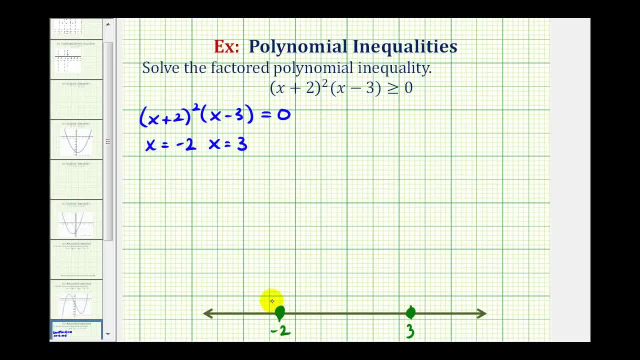 If it does not satisfy the inequality, then the interval is not part of the solution. So let's use the test values of. let's say x equals negative 3 to the left, Let's use 0 in the middle and let's use 4 on the right. 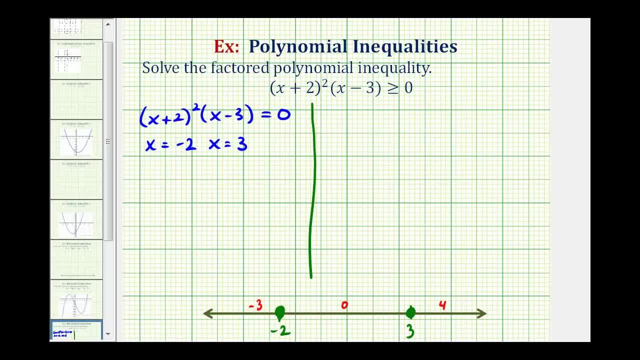 Now we're going to perform substitution into our inequality. So when x equals negative 3, negative 3 plus 2 is negative 1.. So we'd have negative 1 squared. Negative 3 minus 3 is negative 2.. Negative 6,. we want to know if this is greater than or equal to 0.. 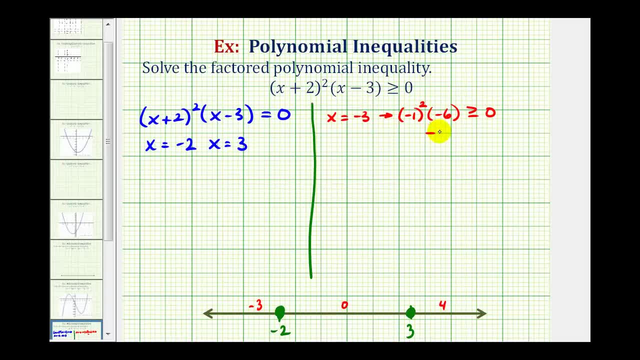 Well, negative 1 squared is 1.. 1 times negative 6 is negative 6.. Negative 6 is not greater than or equal to 0. So this is false, which means the interval on the left here is also false. 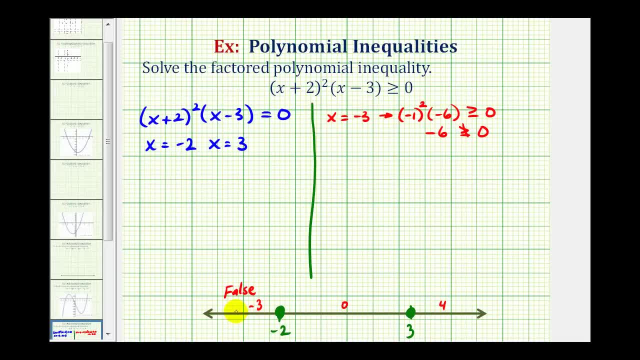 meaning it's not part of the solution. Now I move to the next interval and we'll test x equals 0.. If x equals 0, we would have positive 2 squared Negative 3 times negative, 3, greater than or equal to 0.. 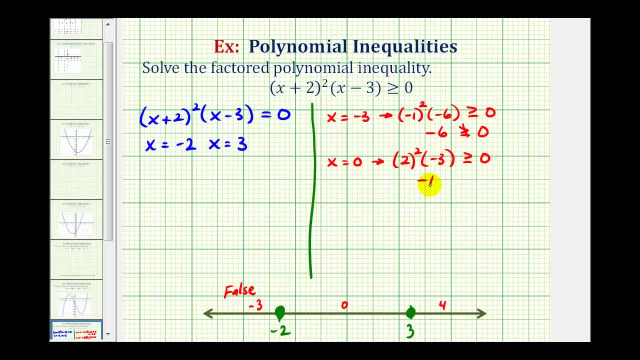 2 squared is 4.. 4 times negative 3 is negative 12.. Well, negative 12 is not greater than or equal to 0. So this is false. So this next interval here is also false, meaning it's not part of the solution. 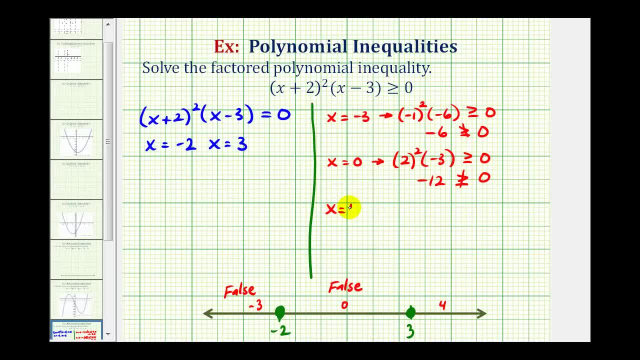 We have one more test value We want to test: x equals 4.. If x is 4, we would have 4 plus 2, or 6 squared, So we'd have negative 4 squared, And 4 minus 3 is 1, greater than or equal to 0.. 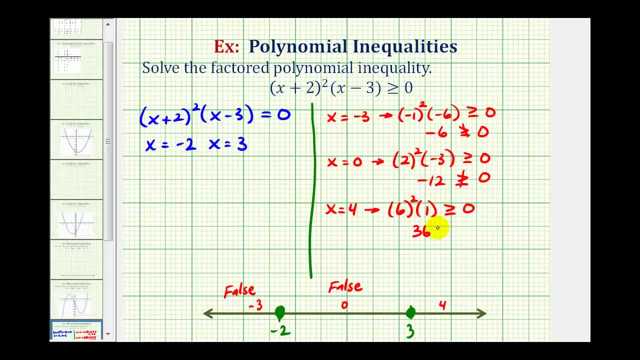 6 squared is 36 times 1 is still 36.. 36 is greater than or equal to 0. So this is true. So if x equals 4 is true, that means this interval on the right is part of the solution. 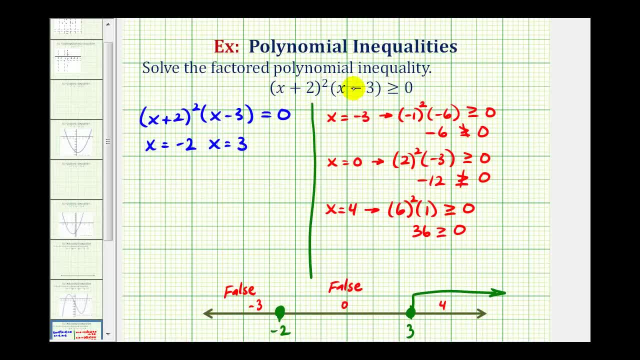 So we'll go ahead and graph this. So the x values that satisfy this inequality is: x equals negative 2, and x greater than or equal to 0.. So this graph represents the x values that satisfy this inequality. but we can also say x equals negative 2, or x is greater than or equal to positive 3..